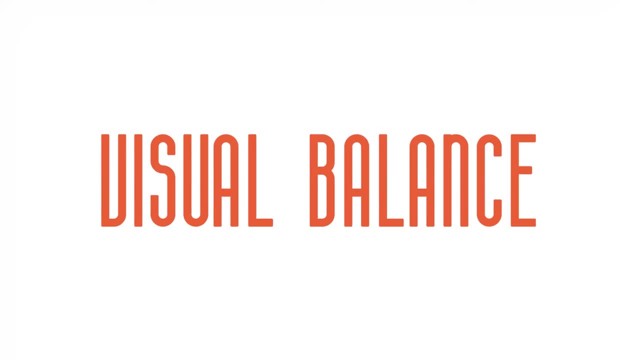 stuff. In order to design icons that look alike, you need to decide on a visual language, make sure the colors match curves, stroke, width, etc. However, that isn't enough. In order to visually balance icons, you need to follow a certain grid. I found this grid. 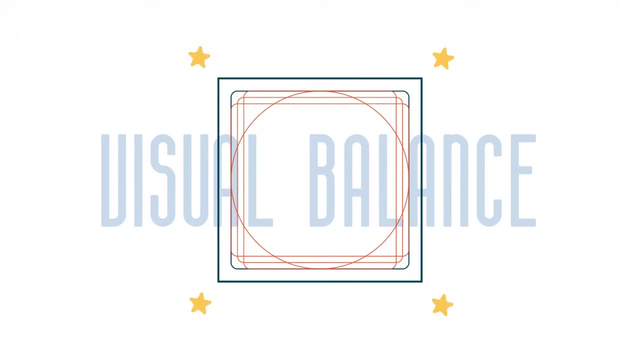 on a channel called Friends of Figma that does tutorials on Figma. Go check them out. link in the description. However, we will be working on Illustrator. Basically, this grid makes sure that the icons look coherent and easy on the eye, If you. 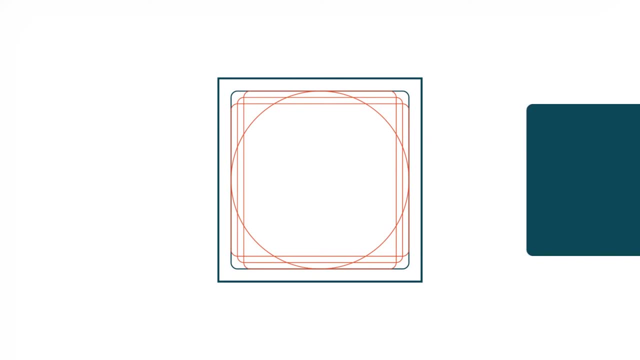 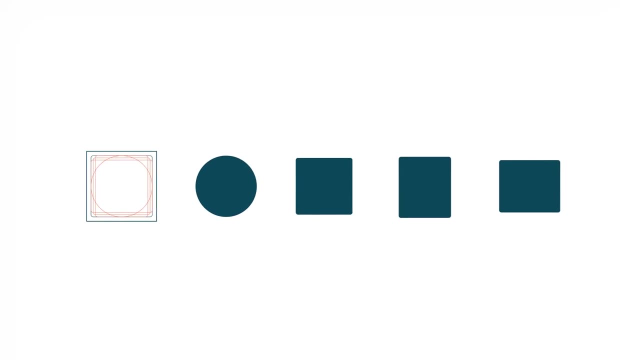 want to design a wider icon, use this rectangular grid. For taller icons, use the upwards one. For square icons, use the square one And for circular icons, use the circle one. Now, if you look at the shapes beside each other, they visually appeal together and no. 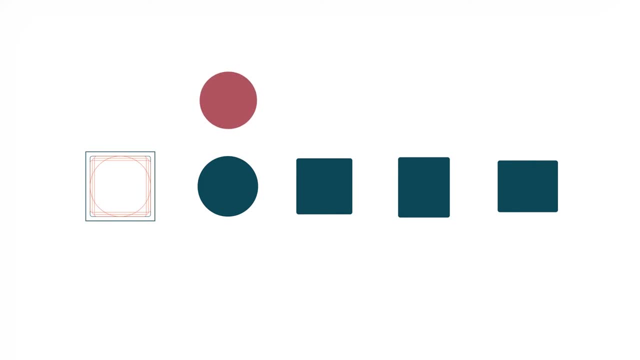 shape feels heavier than the other. In comparison, if you decided to use a circle that is 40 pixels wide beside a square that is also 40 pixels wide, The square that is 40 pixels wide has the same shape and is pixels wide. the square feels much heavier due to the more surface area covered. 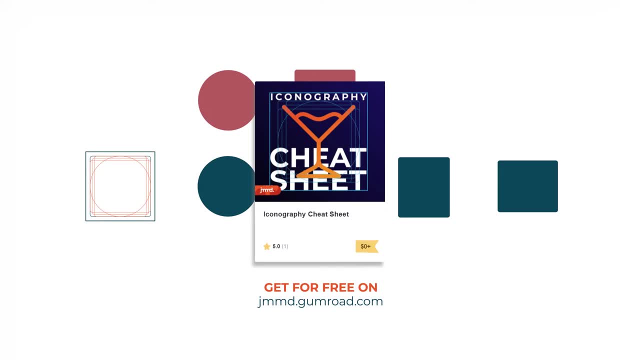 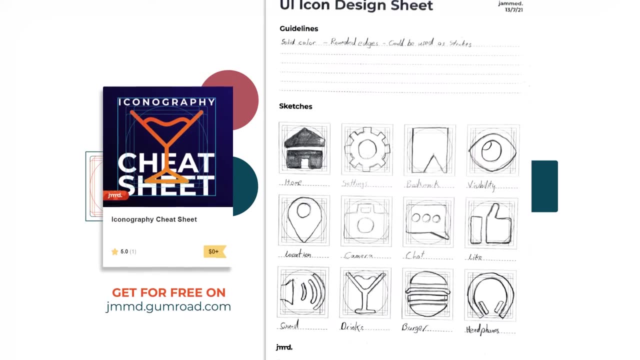 I've uploaded this grid inside of a template on my Gumroad for you to download for free. if you want to design your own icons, I've sketched my own set of icons on an A4 icon design sheet that is also included in the download. 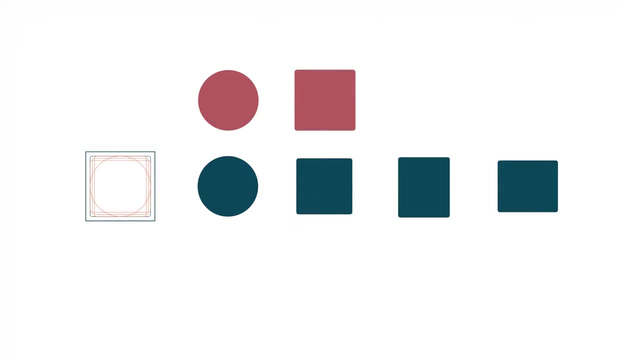 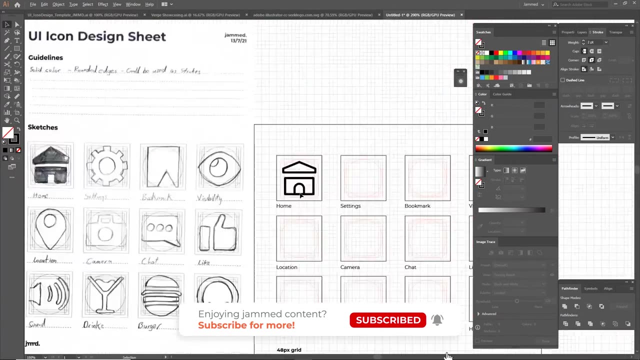 So go get it if you want to design along. Link is in the description. Now that I've finished sketching a set of icons on paper, I'm gonna head on to Illustrator and start applying everything that I've explained, Simplifying the sketches into basic shapes: single stroke width, single color. 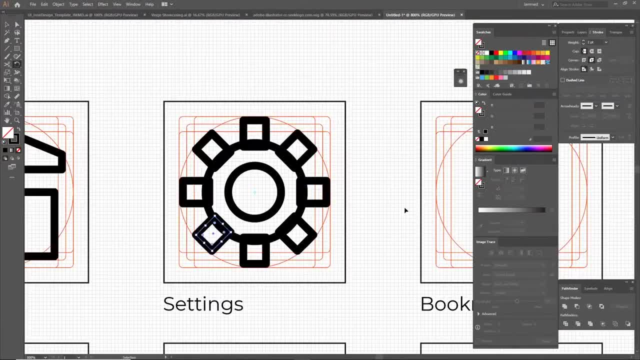 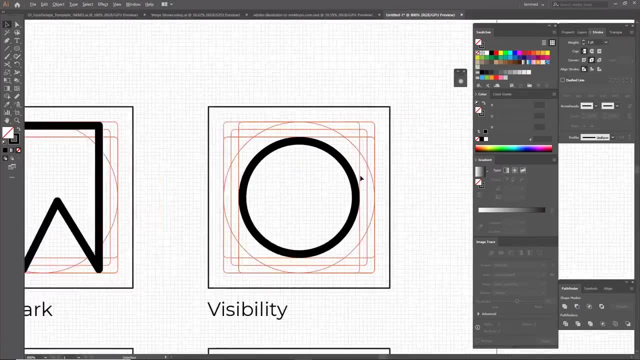 This is a great exercise for all designers out there, and it's actually pretty calming too, Deconstructing anything into basic shapes. I have fast forwarded this video in order not to bore the crap out of you. If you want the full video uploaded, let me know and I'll put it on Gumroad. 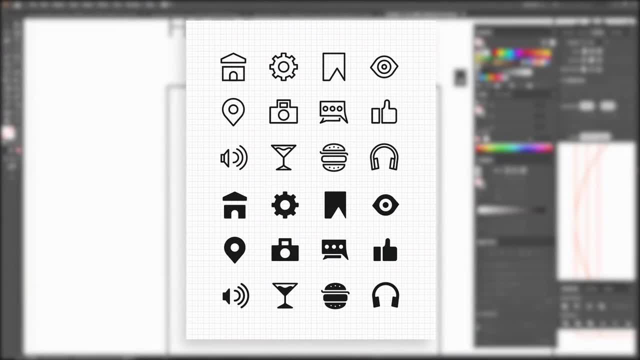 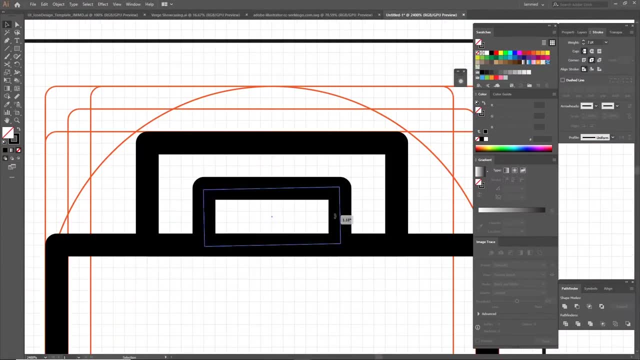 After you're done designing the icons, you can also change them to solid color instead of strokes, and vice versa. This is how you should design icons that really work well together. If you want to make sure of how your icon looks at a certain pixel size, make sure your 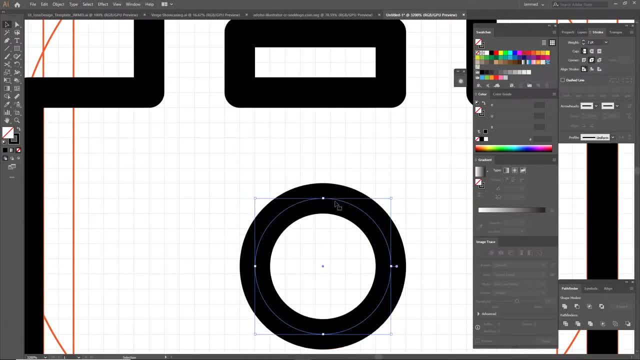 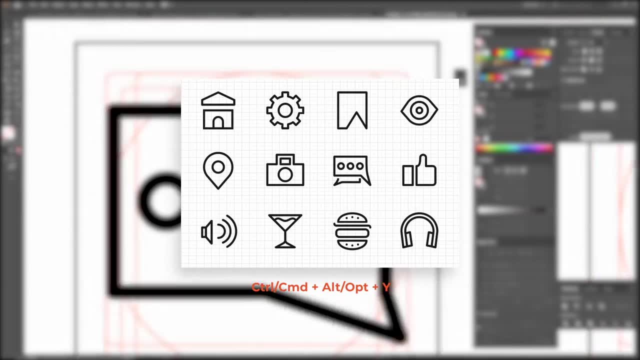 icons are at the ideal pixel size you want it to be, And press Ctrl-Alt-Y on Windows or Command-Option-Y on Mac, which turns on pixel preview. This lets you see how your icons really look like on screen once they're rasterized. 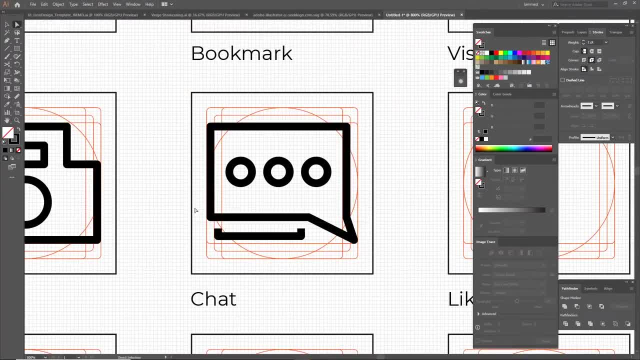 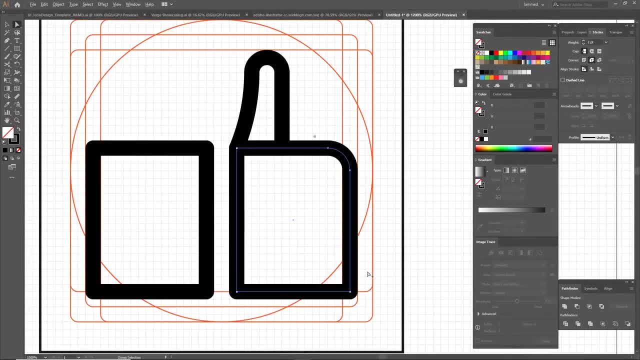 This way, you can judge whether you can adjust it to look better on pixels or leave it as it is. It is important to know the size of the screen you're designing on and the size of the icons on the screen before designing them, because then you won't need to re-iterate them as